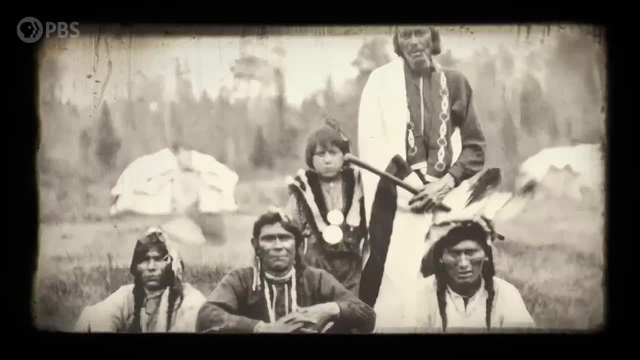 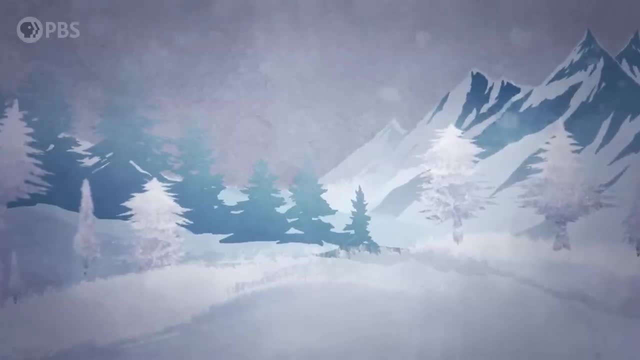 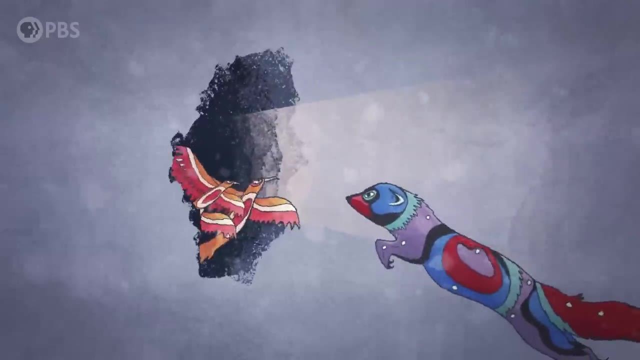 knowledge was encoded in myths. The Ojibway people native to the Great Lakes region in the US tell a myth about the Fisher constellation. Long ago, the world was covered by snow and ice and there were no birds to announce the coming of spring. The Fisher was a great hunter who went up to skyland. 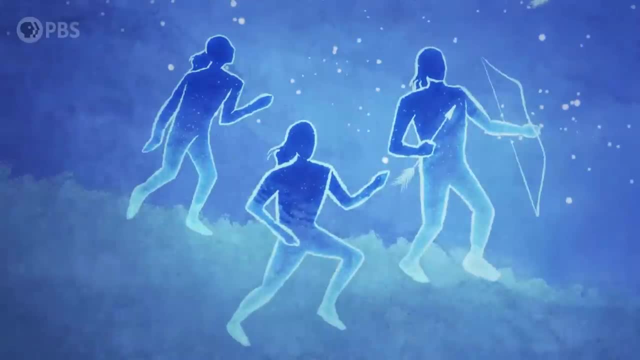 to free the birds and bring warmth back to the Earth. When the sky people caught Fisher freeing the birds, they began chasing him. When the Sky People caught Fisher freeing the birds, they started to chase him, but it was not enough. They expected that a man or woman. 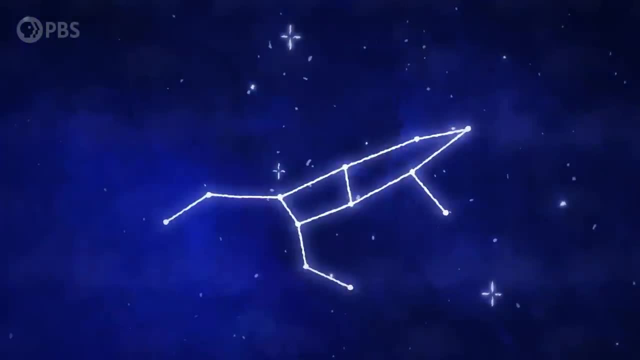 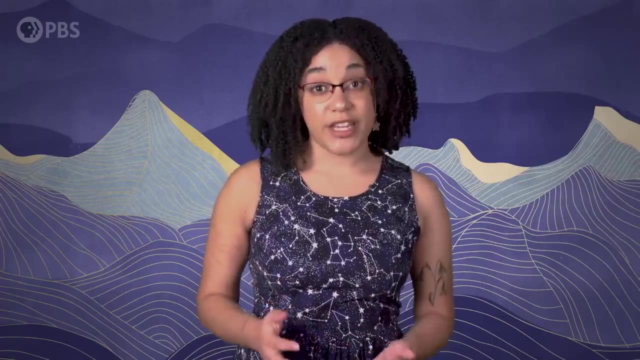 but he escaped to the sky, where he was trapped forever by an arrow through his tail. This Ojibwe myth serves multiple purposes: It explains the changing of the seasons, and the constellation it's attached to acts as a reminder of spring's return. 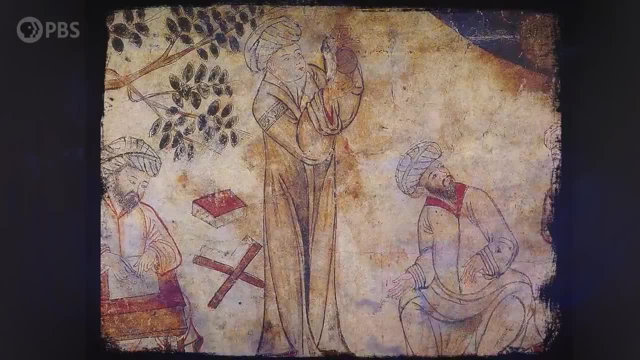 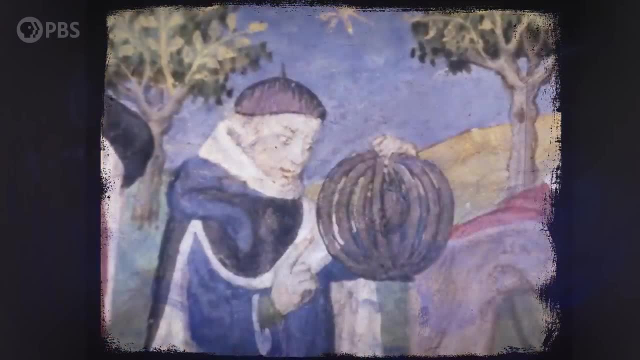 No matter what they used the constellations for, the fact that ancient humans used them at all meant that people were studying the sky. The brightest minds around the world took meticulous notes about how the sky changed over time. and without those early astrologers, 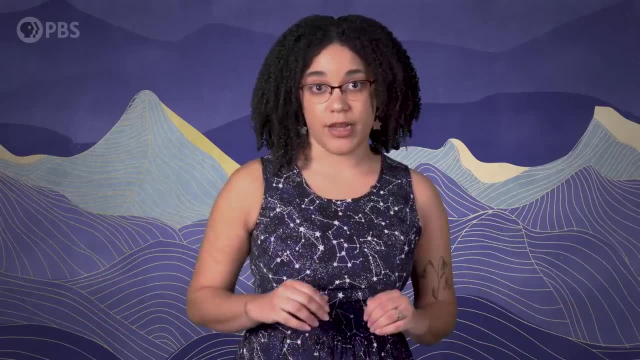 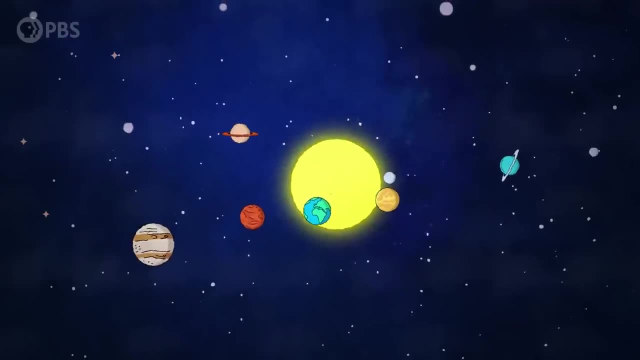 the field of astrophysics as we know, it would be drastically behind. I would probably lose my astronomer's card if I didn't tell you this at some point. so here goes: Our planet is just one of many orbiting a star which is just one of billions. 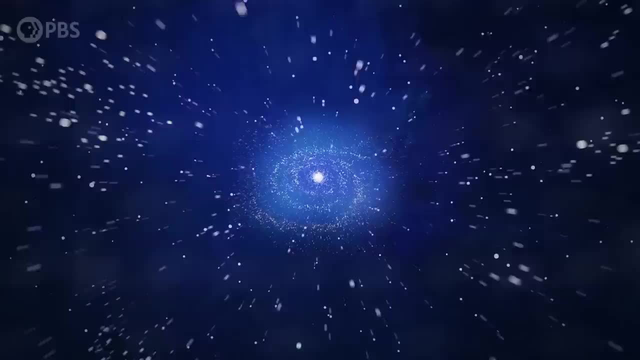 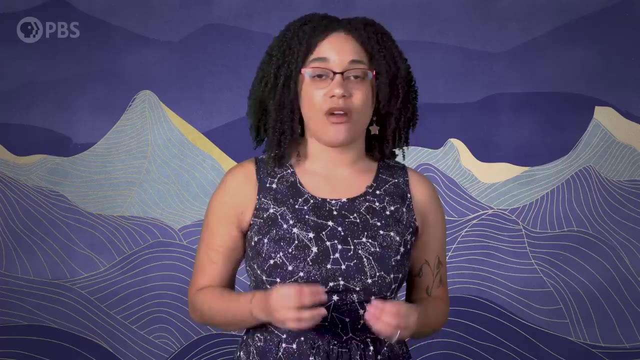 orbiting a galaxy which is itself also just one of billions in the vast universe. The points of light that we see in the sky are distant stars and, despite what the myths may tell us, their arrangement is nothing more than a coincidence Based on early written records and physical artifacts. 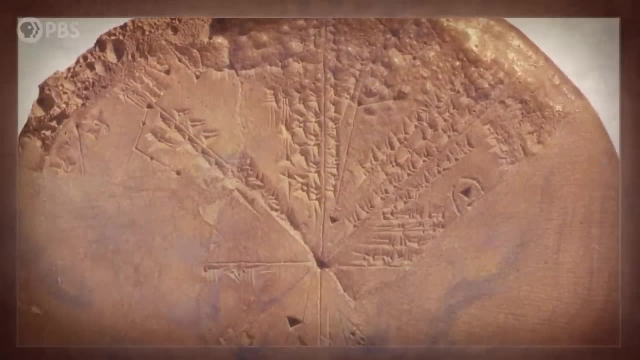 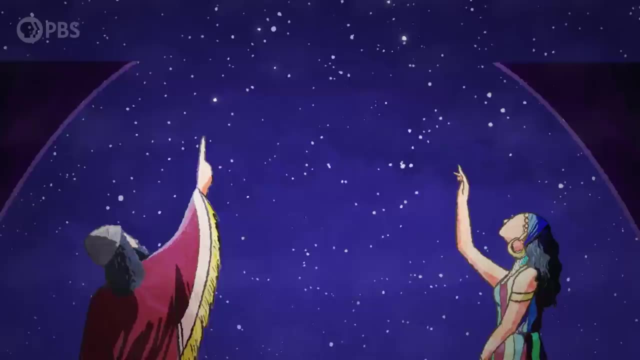 most historians agree that ancient Mesopotamians were among the first to observe the motion of stars in the sky and assign divine meaning to it. Because the sky was believed to be the home of many gods, the shifting shapes in the inky darkness were interpreted as omens. 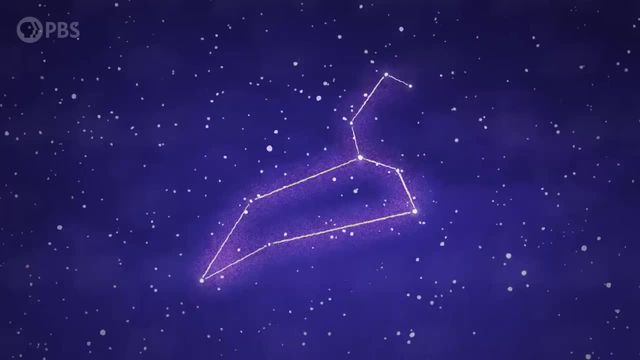 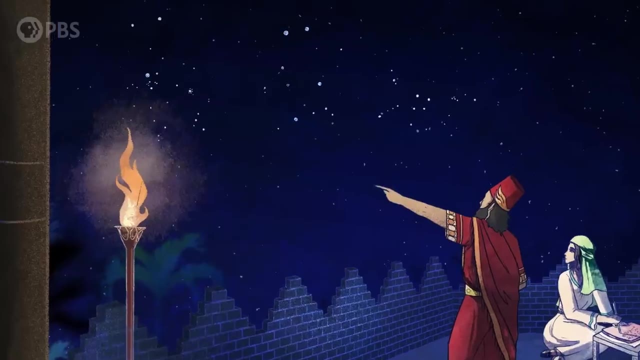 like an omnipotent teacher scribbling on the blackest of boards. Babylonian skywatchers in the 18th century BCE were especially prolific in their study of the heavens. The Babylonians and their neighboring Assyrians also gave us many of the constellations. 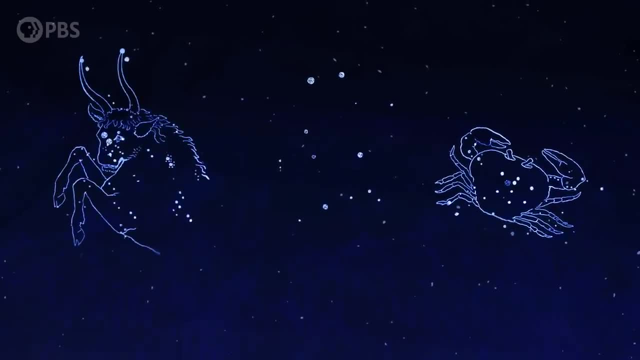 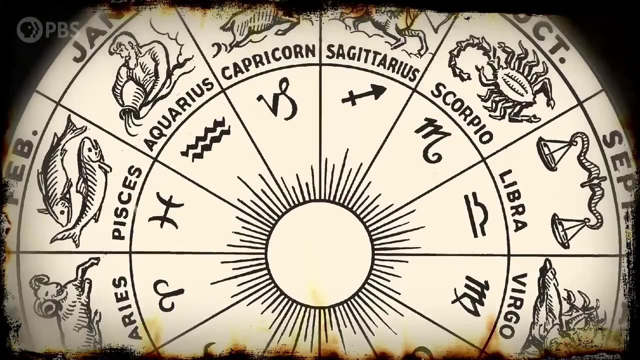 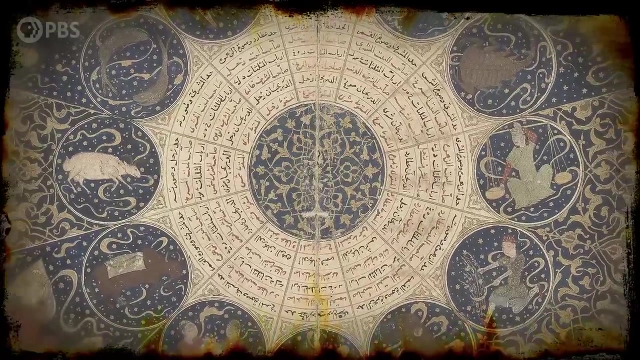 we use in the West today, like the crab, the bull and the twins, but we would call them cancer Taurus and Gemini. Ancient Mesopotamians even invented the zodiac, the sequence of 12 or 13 constellations that the sun appears to pass through over the course of a year, though the 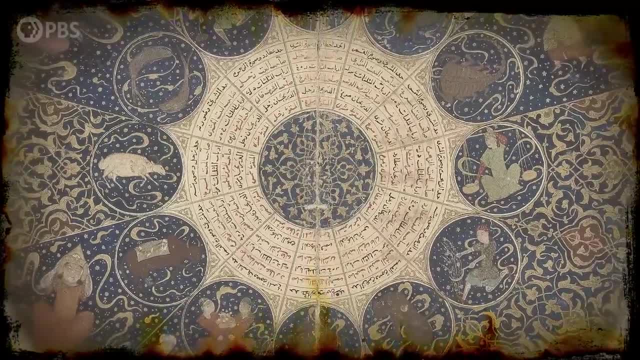 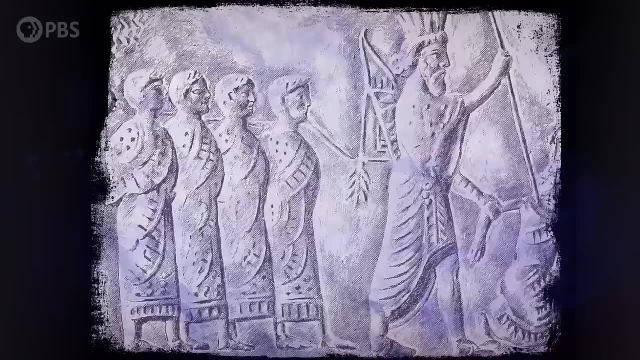 sequence's name and its association with horoscopes were added by the Greeks almost two millennia later. Originally, the zodiac was used as a way to keep track of time. The Mesopotamian constellation myths have some interesting meanings. They are often used to describe the time of a planet, but the 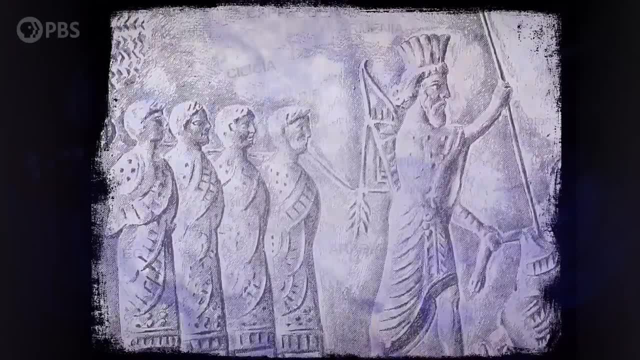 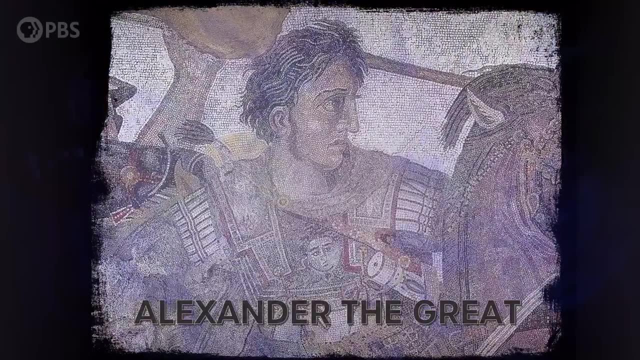 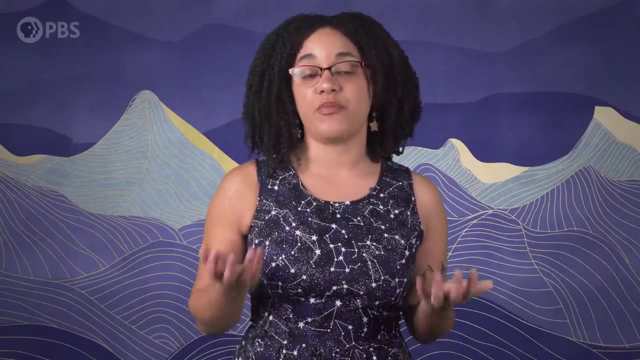 trickled into Egypt over a few hundred years after it was conquered by Persia and then Alexander the Great. in the 6th and 4th centuries BCE. These new myths merged easily with the Egyptians existing beliefs, because they had already been using the patterns of the night sky to keep track of time for 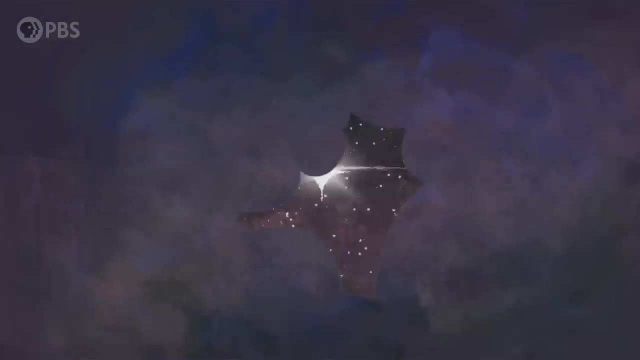 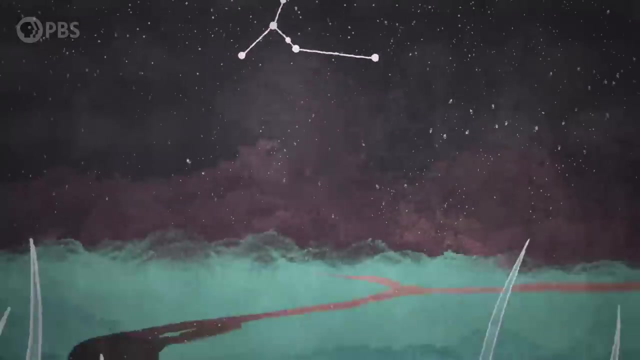 practical reasons, most of them having to do with farming. When Sirius, the brightest star in the sky, appeared over the horizon, ancient Egyptians knew that it was almost time for the Nile River to have its annual flood, which would nourish the soil for the next year's crops. The constellation mythology spread. 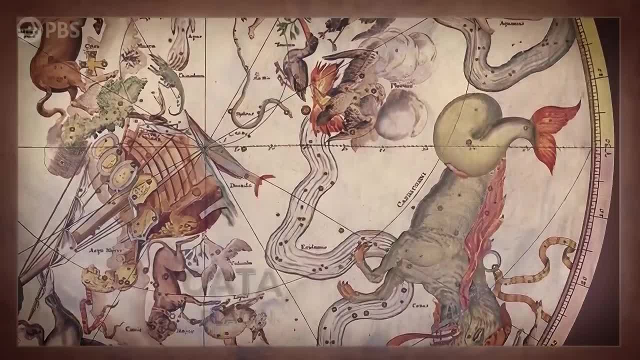 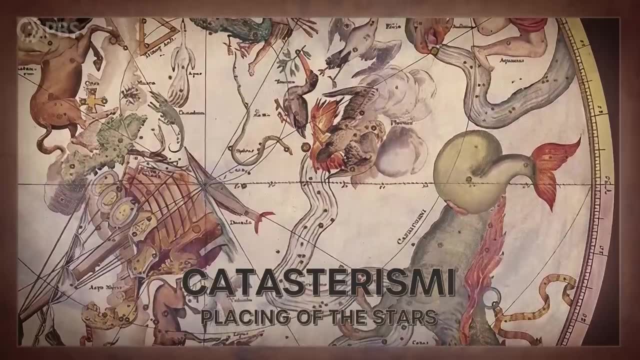 to Greece by the 3rd century BCE, where they were called katasterizmi, meaning placing of the stars, because they believed that the constellations were put in the sky purposefully by the gods. to teach them lessons, The Greeks'. 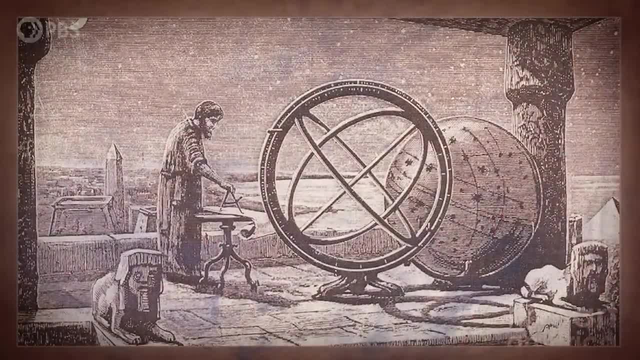 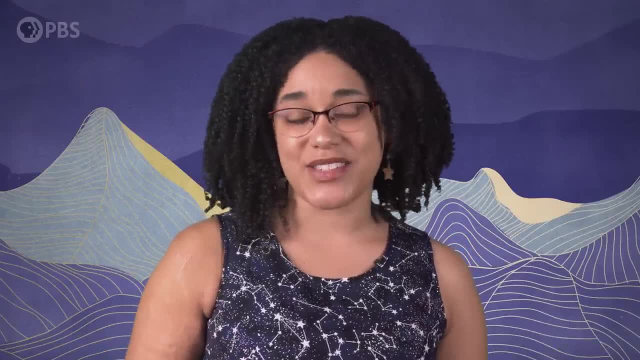 religious fervor, combined with their taste for numbers, produced astronomy: the meticulous and mathematical observation of the sky. You know, you know, you know, so that we can know exactly how the gods want us to live our lives. Unfortunately, Greek astronomers, like Ptolemy, spent all that effort describing 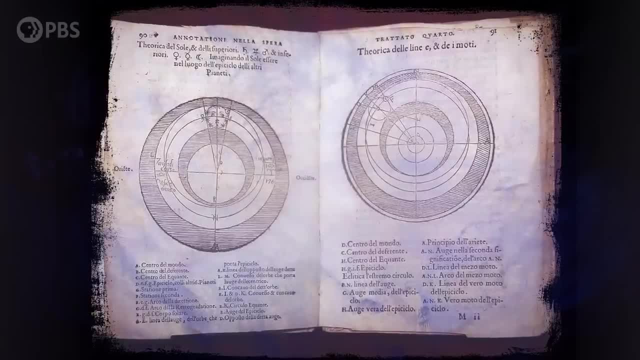 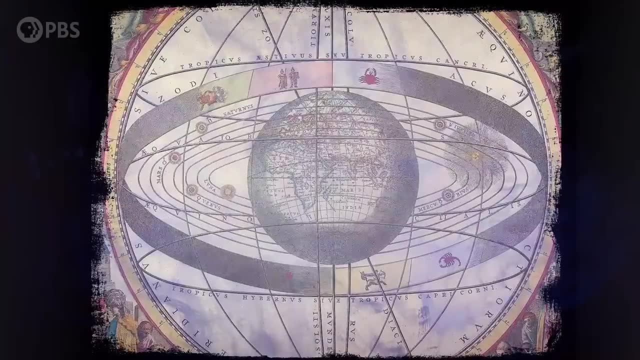 a system that relied on a fundamentally flawed assumption. They believed the Earth was the center of the universe, and that belief held as both astrology and astronomy made their way through the Islamic world and over to Europe, where geocentrism remained popular until the heliocentric revelation in the 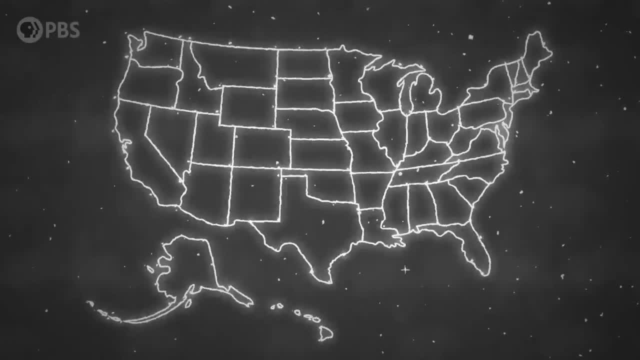 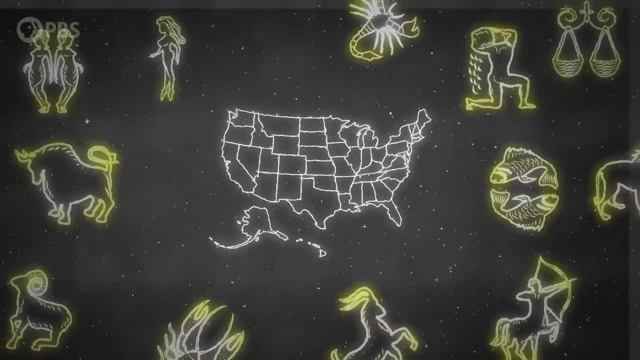 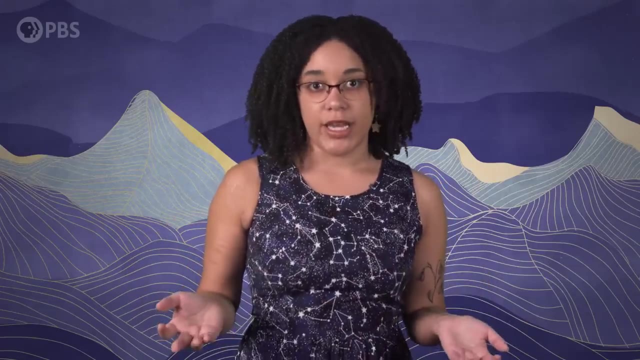 1500s. Nowadays, around 70 million Americans claim to read their horse every day, and nearly a third believe that astrology is real or vaguely scientific. As a scientist, I don't love those stats, but astrology in western countries is mostly a novelty. 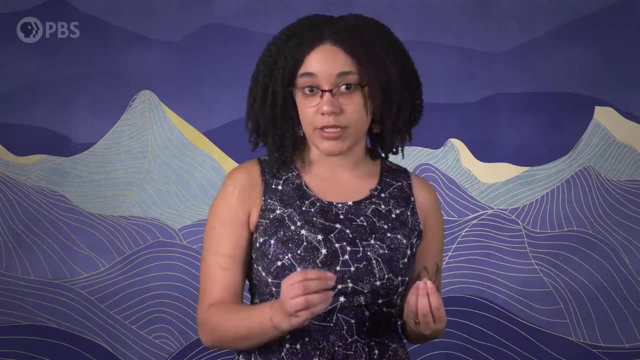 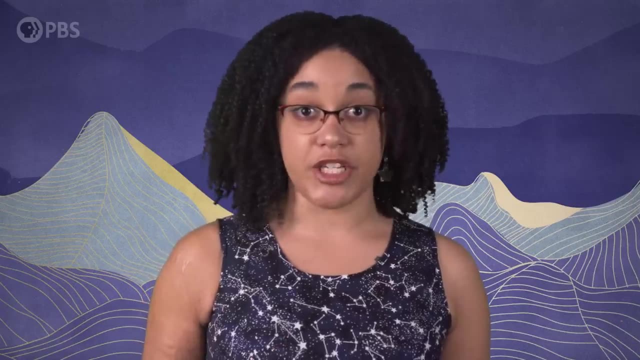 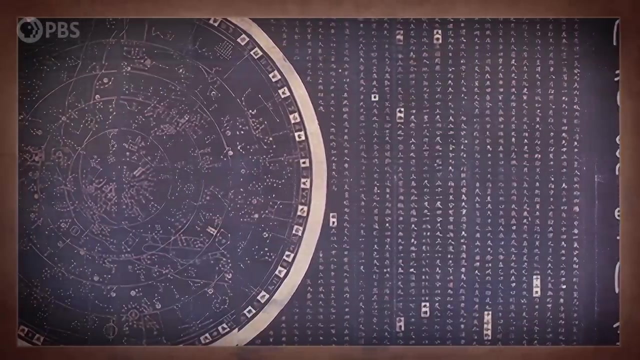 an interest that people might use to help them make small decisions, But different astrologies developed more or less independently in China and India, each with their own constellations and interpretations. Astrology is still popular in some parts of the east, like in China, where star charts may. 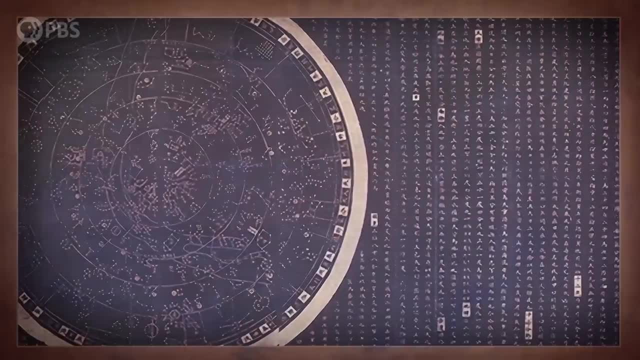 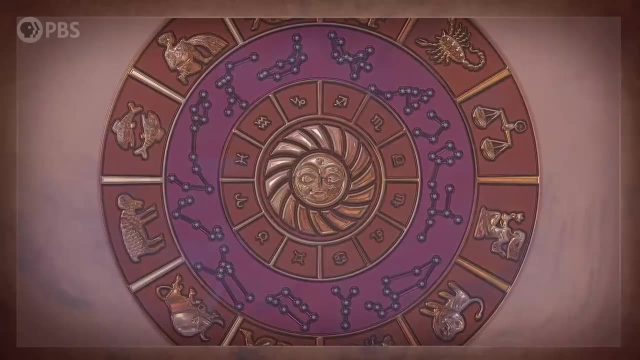 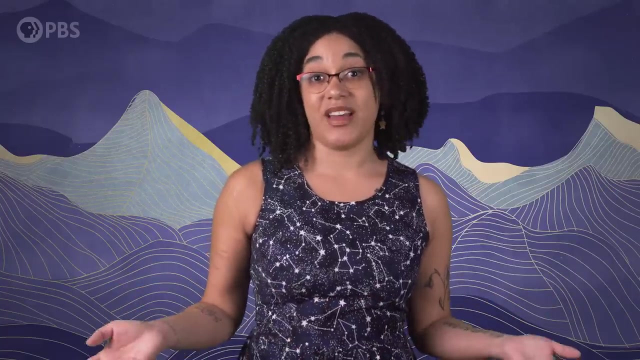 be consulted to determine compatibility and love or to make a big career decision. In India, astrology is used by many to dictate decisions about medicine, marriage, careers, business deals, often in a harmful and discriminatory way. I've always thought it was kind of a shame that conversations about constellations are so often. 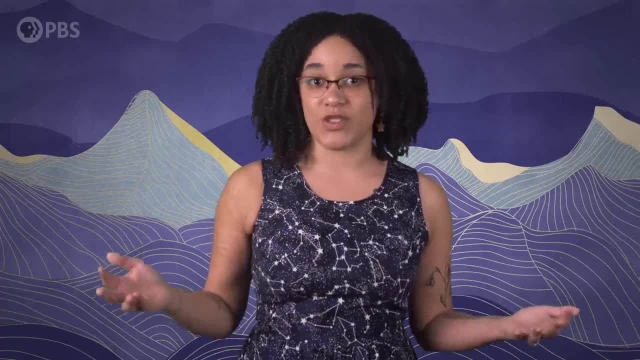 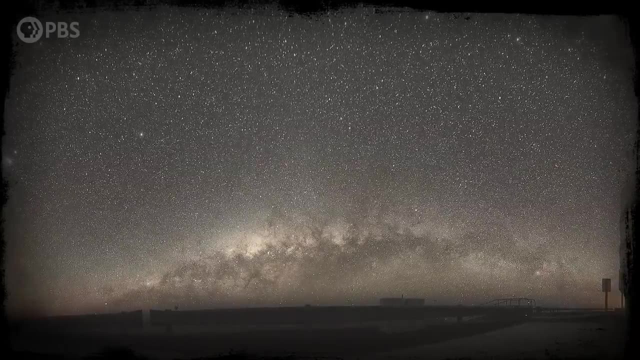 dominated by the Greeks. because some of the most beautiful views of space can only be seen properly from the southern hemisphere- You can see the blurry Magellanic clouds and the dark rift cutting across the stream of the Milky Way- And because the stars you can see depend on your 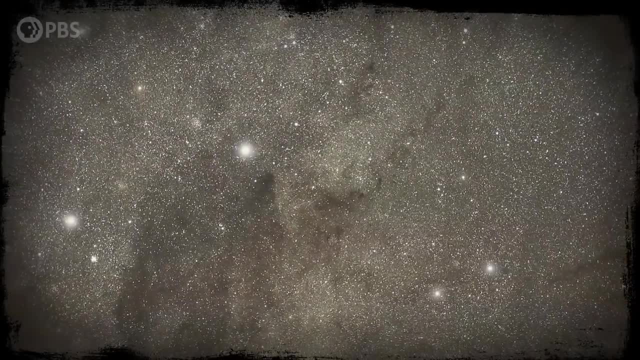 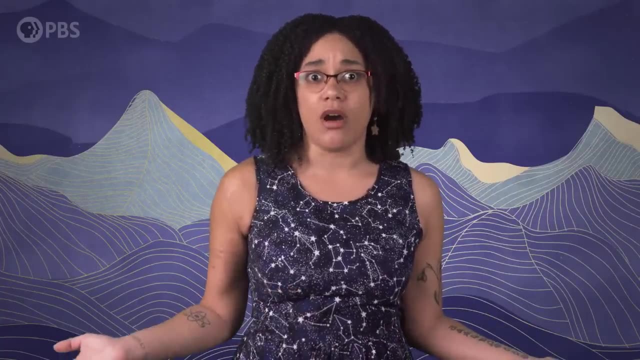 latitude. you can even see different constellations like the Southern Cross. Celestial navigation in the southern hemisphere is inherently more difficult than in the north, because there's no south star that stays put as the rest of the stars appear to twirl around it. 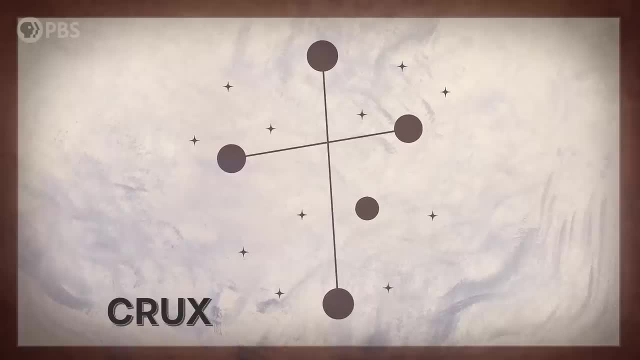 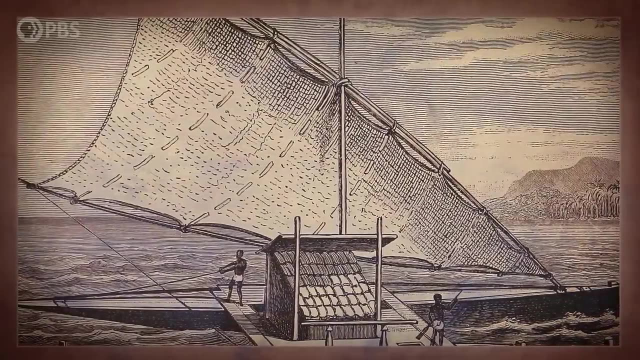 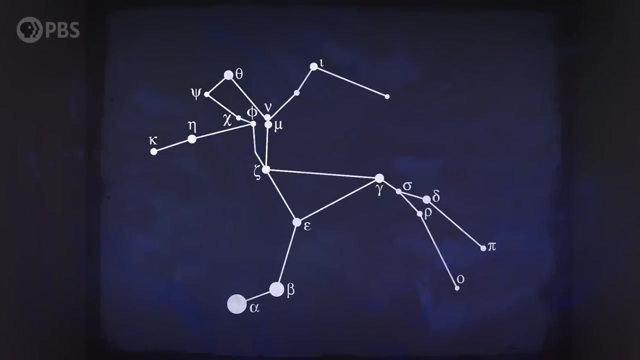 Instead they have the Crux, a small group of four stars. Despite this difficulty, Polynesian wayfarers used the southern stars to travel around the Pacific Ocean more than a thousand years In the time of ancient Greece, before Polaris was our north star, the Crux was visible from more. 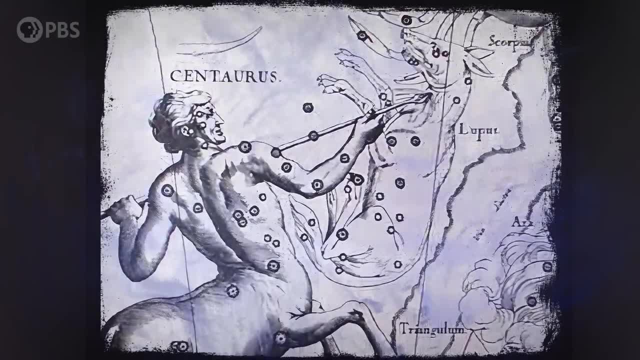 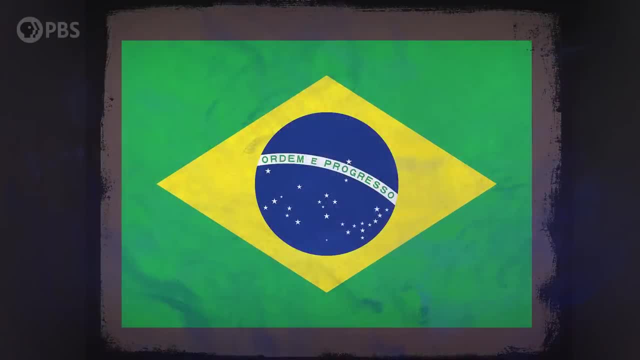 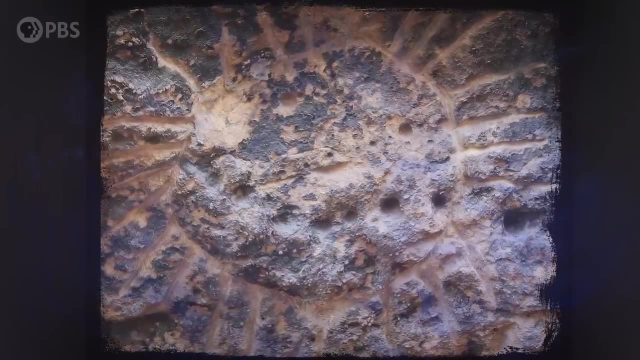 northern latitudes, But the Earth's axis wobbled, and now the Crux is a quintessentially southern constellation, one that features on several southern countries' flags, like Brazil, Samoa, New Zealand and Australia. Some scholars believe that the astronomical record in Australia goes back 65,000 years. 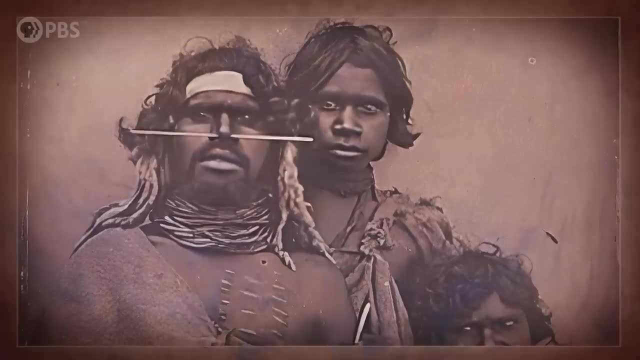 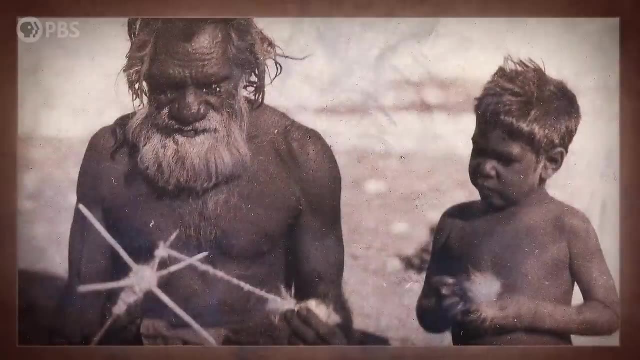 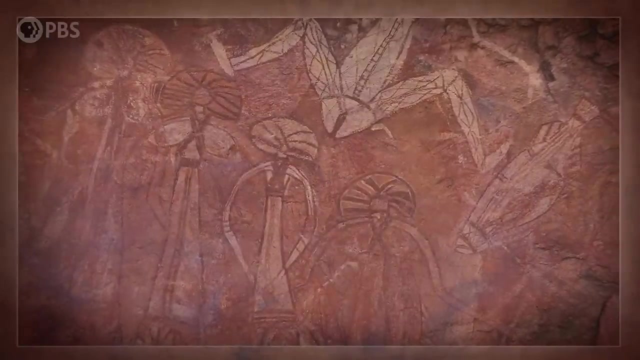 but the timing is hotly debated. The Aboriginal and Torres Strait Islander people are spread between several hundred different language groups with a wide variety of spiritual beliefs and lore. Despite their many cultural differences, cave paintings and even other archaeological evidence show that many Aboriginal Australians were using stars as calendars for more than 10,000 years. 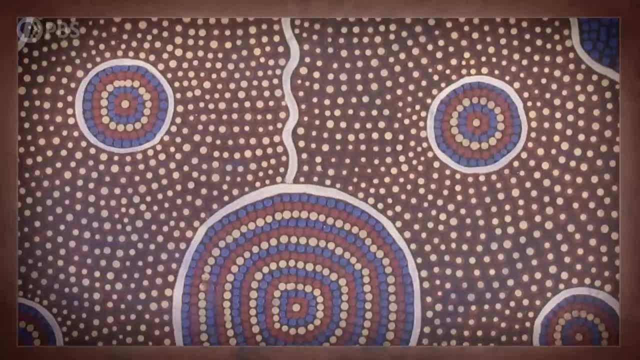 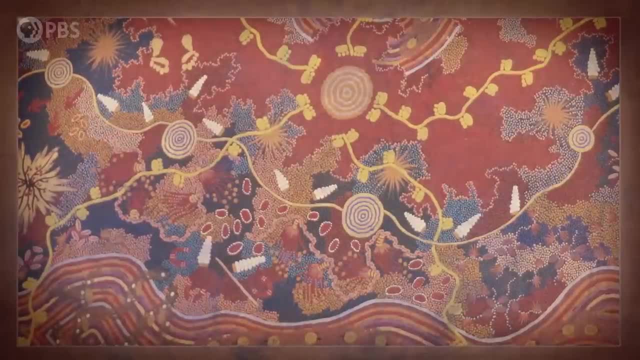 before the Babylonians read their motion as omens, In a time before written language was developed, the city's irregular infrastructure- minus life бы تчто—, these celestial timekeepers- was passed down through oral stories and other art forms. One constellation common to many of the Aboriginal cultures is the Emu. 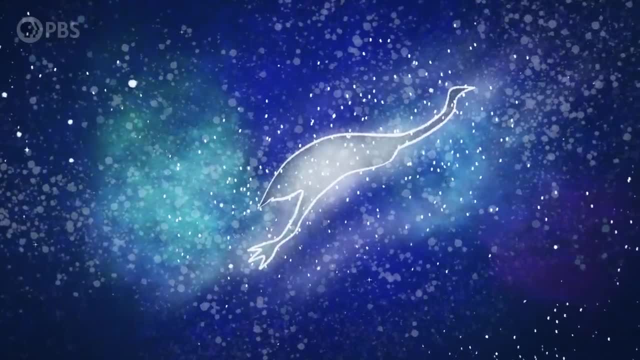 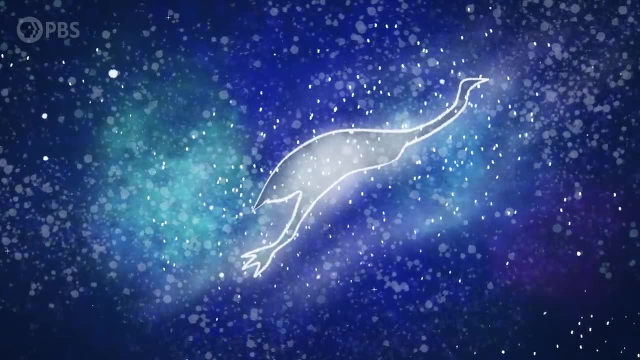 whose head was the dark Coalsack Nebula, nestled next to the Southern Cross. The Emu's legs stream out behind her and some stories say this is because the Emu used to have great wings, that it used to fly across the sky. The Emu- 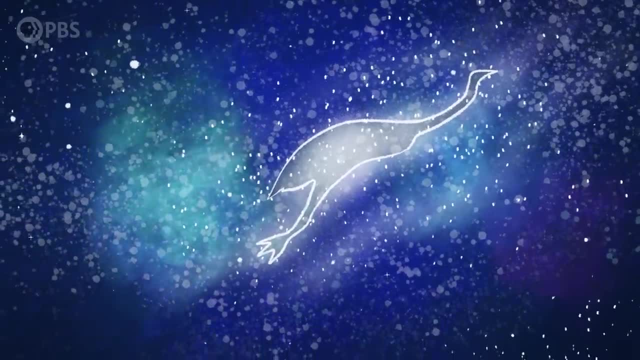 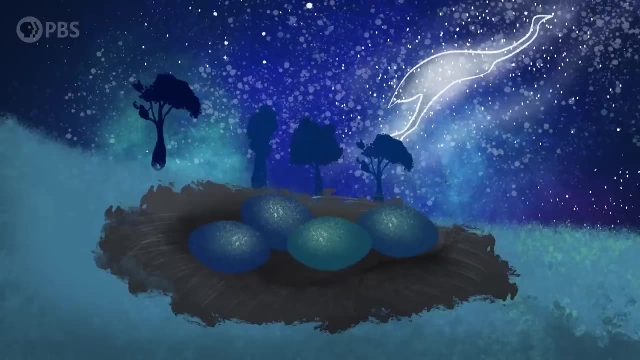 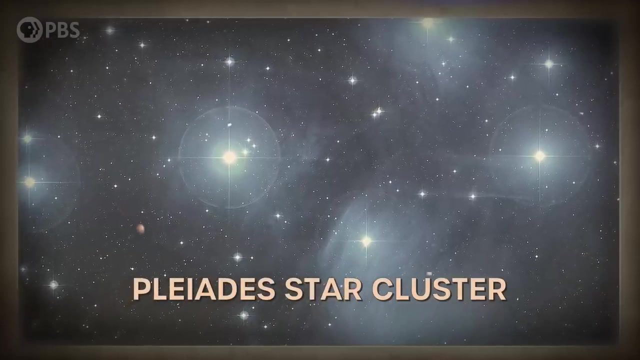 constellations appearance in the sky coincided with egg laying season for the more earthbound Emus. Those eggs are an important source of nutrients for the Aboriginal Australians, and so the constellation was a life-saving reminder. The Pleiades star cluster is known among many groups as the Seven Sisters, Though 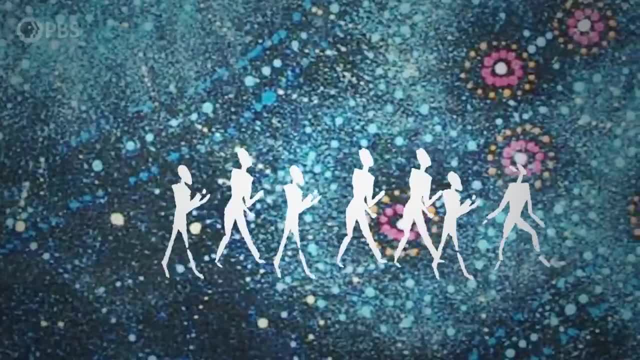 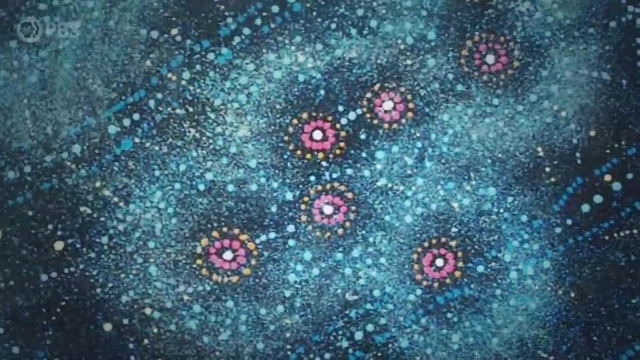 the details of the story vary across the continent. the sisters are usually said to be running from something, maybe a hawk or an unwanted suitor. The Yamaji people in Western Australia used to predict how heavy the seasonal rains would be, based on how bright or warm the weather would be. 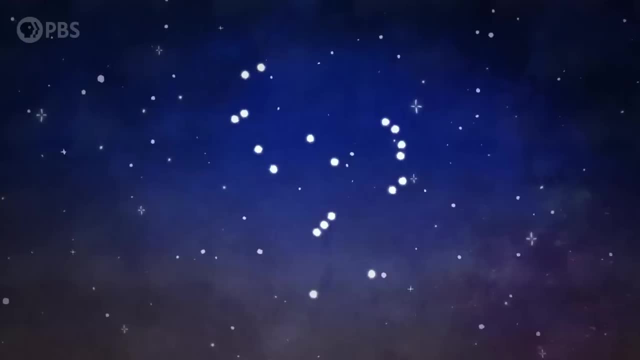 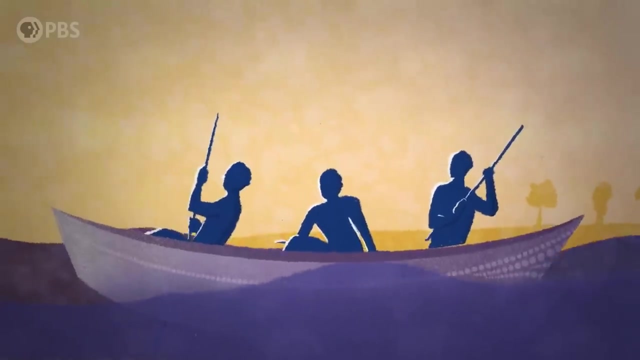 To some Aboriginal cultures, the stars in the western constellation Orion form a canoe. according to the Yolngu people in the Miwat region of Northeastern Australia, The three stars that make up Orion's belt represent three brothers fishing in the canoe When one of them got hungry enough to break the law by eating. 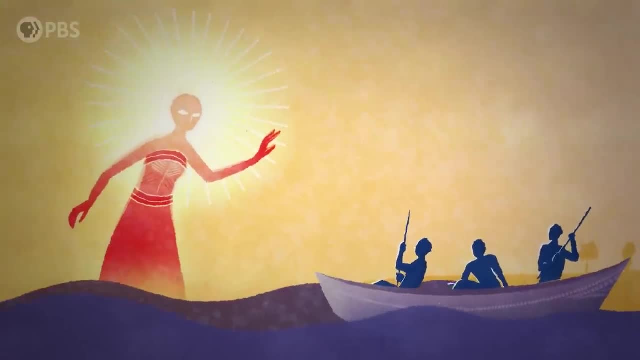 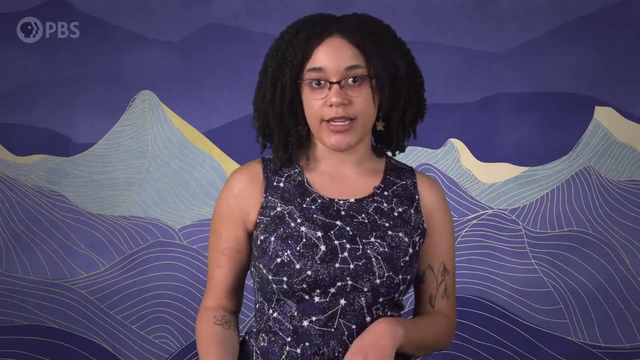 a sacred fish, Waloo. the Sun Woman lifted them to the sky in punishment. So ancient humans all over the world used the sky to: to learn and teach traditions, to navigate and keep time. Unfortunately, so many people today are prevented from connecting to the stars. 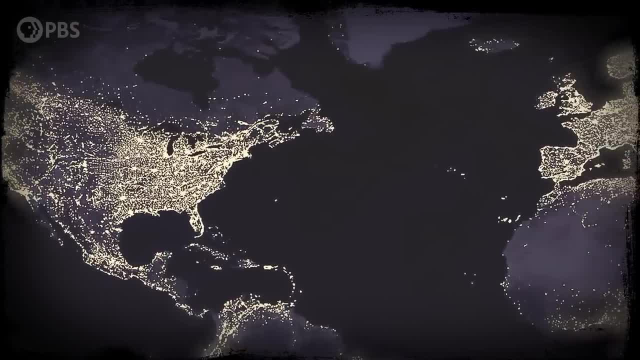 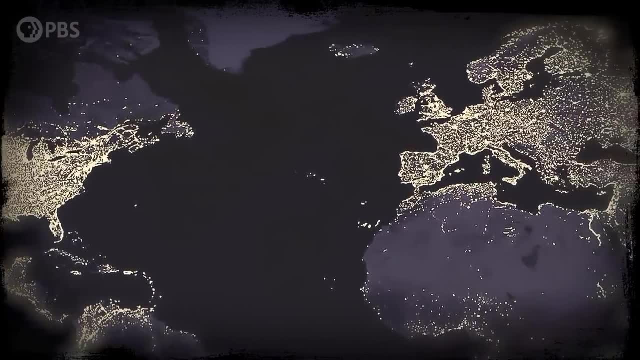 in the same way our ancestors did. According to the Dark Sky Association, a nonprofit dedicated to ensuring that everyone has access to the night sky, about 80% of the world's population has a diminished view of the sky because of light and air pollution.